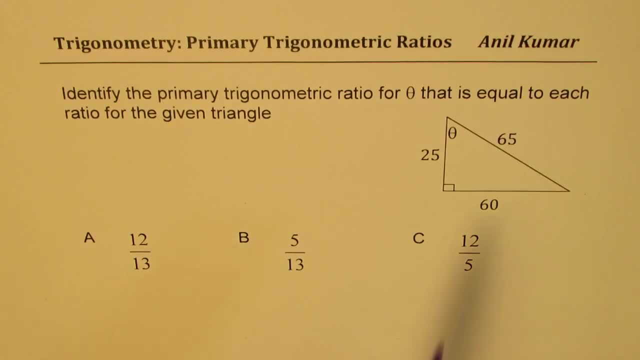 The last question here is to match. We are given the angle theta and some ratios here. Now these are. these could be matched to trigonometric ratios: sine theta, cosine theta and tan theta. So that is the last question for you. You need to match these ratios, Perfect. 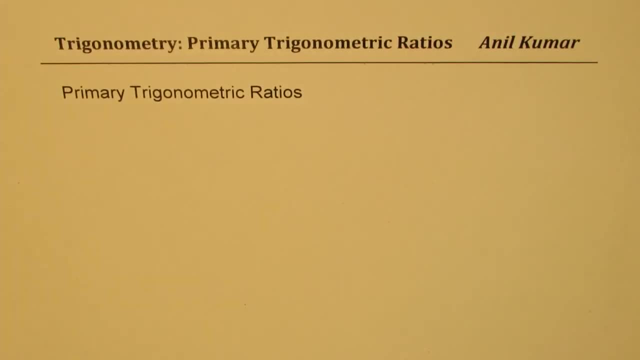 Now let us see how to solve such questions, right? So we will begin with basic primary trigonometric ratios in a right triangle. So let me sketch a right triangle here. So in any right triangle, Pythagorean theorem is always true, that you know, right? So let us say this, right? 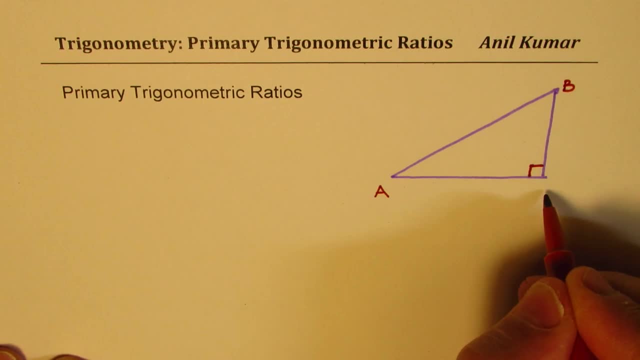 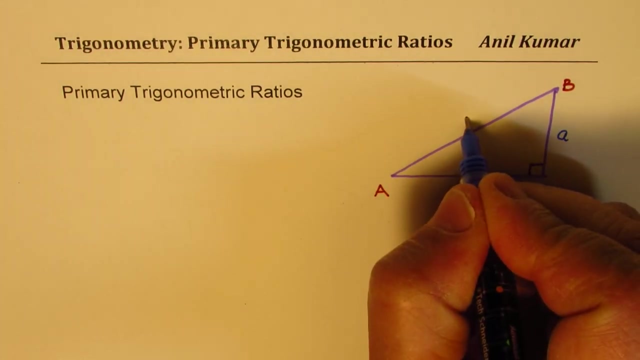 triangle is AB and C. Now the sides opposite to A normally will be written as lowercase A, opposite to B will be written as lowercase B and opposite to C will be written as lowercase C. So from Pythagorean theorem we know one thing that is: 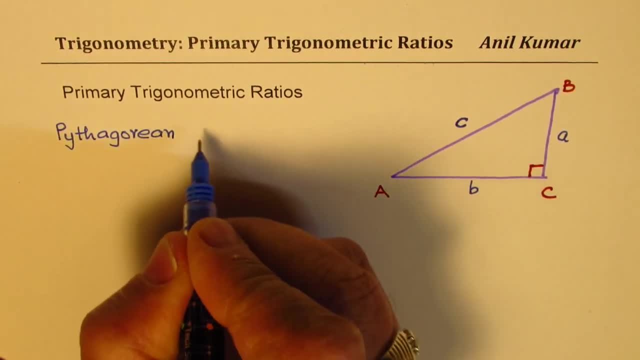 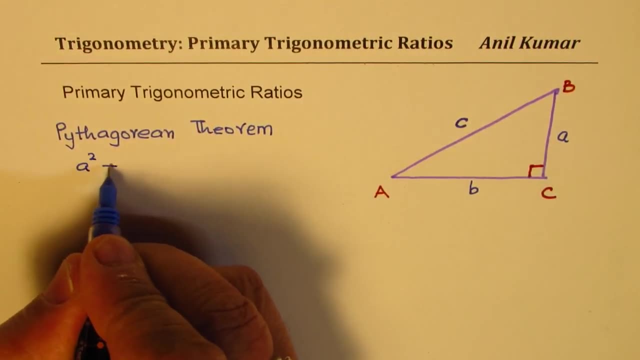 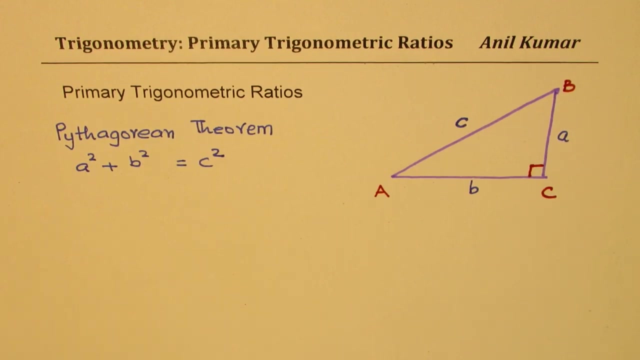 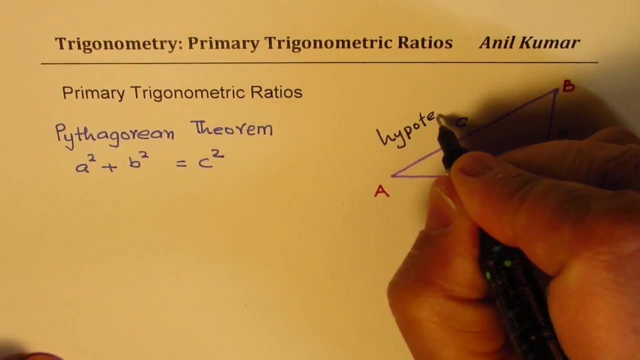 All these sides are related, right? So from here we know: A square plus B square is equal to C square. Longest side in this particular case is called the hypotenuse range. So let me write down hypotenuse here. Let us say we consider angle A. So let us say angle. 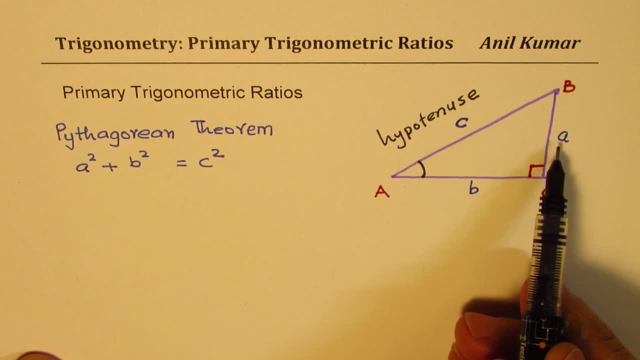 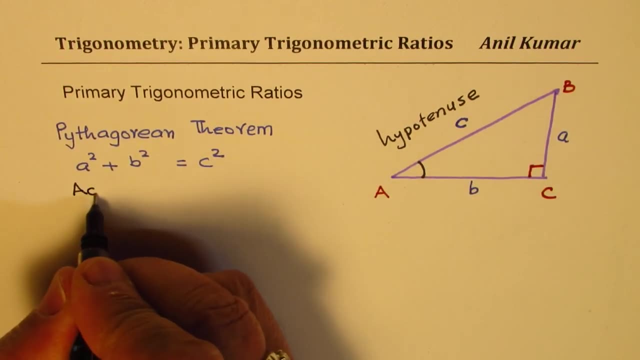 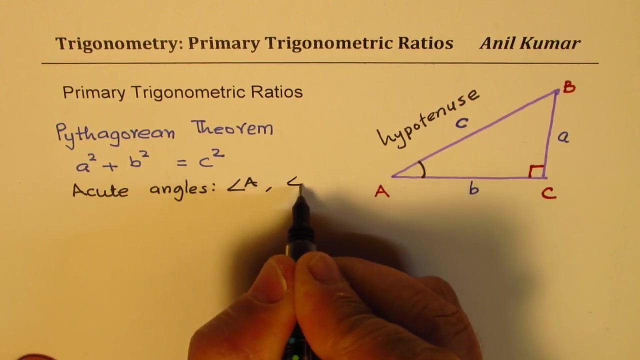 A. So let us write down hypotenuse here. So let us say we consider angle A. So let us say this value B. Also let us say B, So angle B is the shortest side. So if you look at this diagram here, we have only one triangle, right. 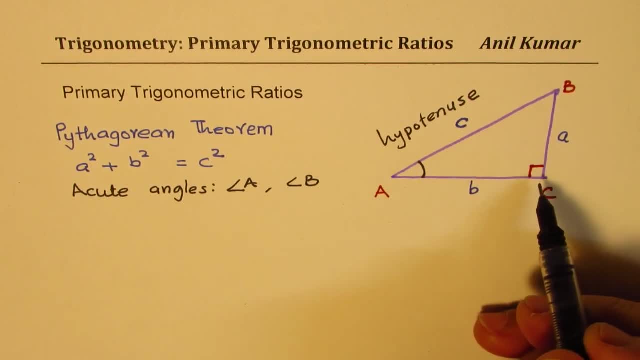 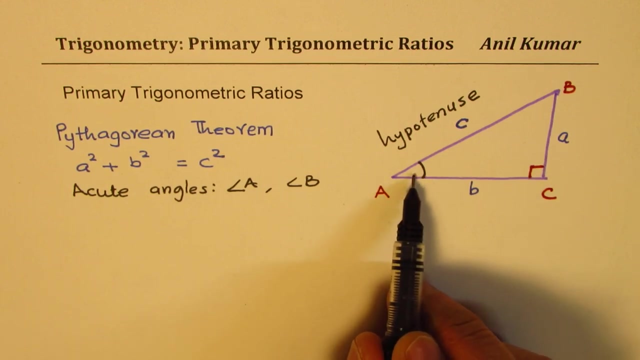 What else is there? The next angle we need is the diagonal angle. So when we, Dracula Drei, tells us that always, under root, N is equal to 90,, we are actually losing 90. See this: acute angles. Now considering angle A, the side which is between the angle and the right, 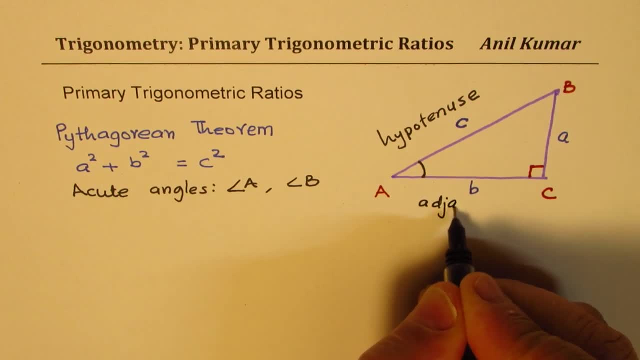 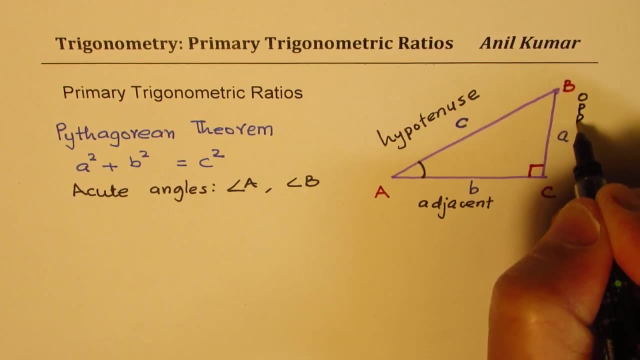 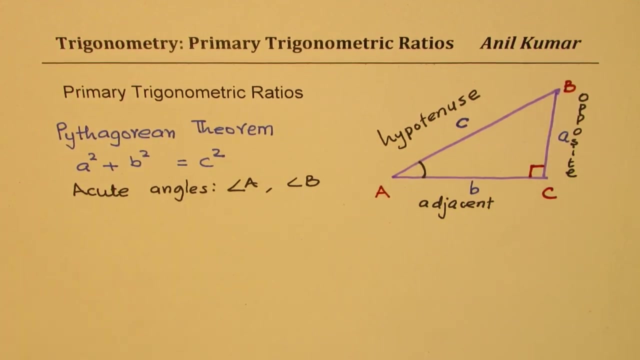 angle is termed as adjacent side And this side is opposite to A and we'll always call this as opposite side. So that is how these sides are termed right. So opposite means you're looking from the angle we're talking about, so it is on the other side, far away. 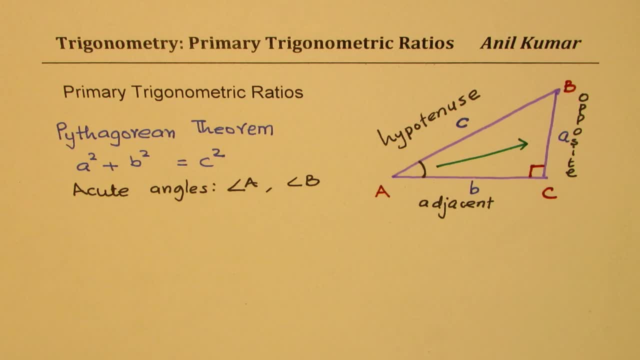 Adjacent is close by correct, So that is another way of looking into it. The ratios which are primary trigonometric ratios are called sine, cosine and tangent. In short, we always write them as sine of an angle. So sine of an angle. in this case I'll write with respect to A. 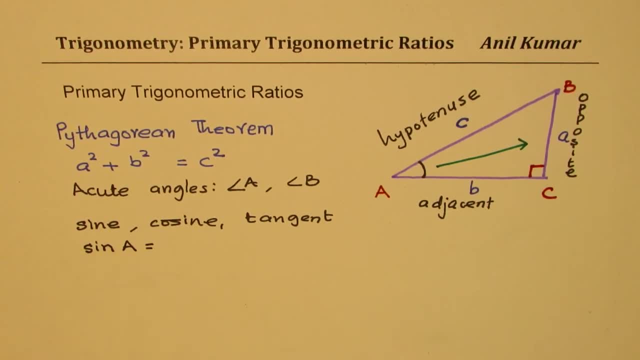 So sine of an angle A right. So this ratio sine A is the ratio of opposite side to hypotenuse. In short, I'm writing opposite side over hypotenuse, The ratio cosine, which in short is written as cos C-O-S. so cos of angle A is equal to. 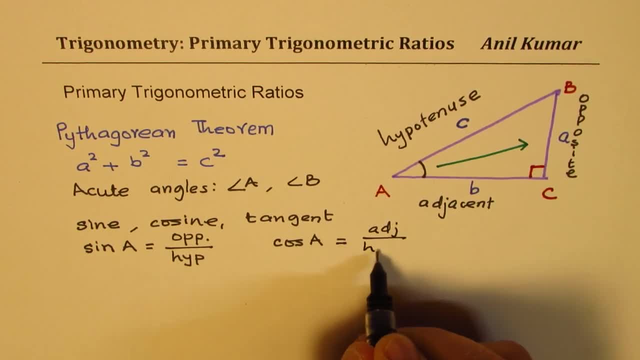 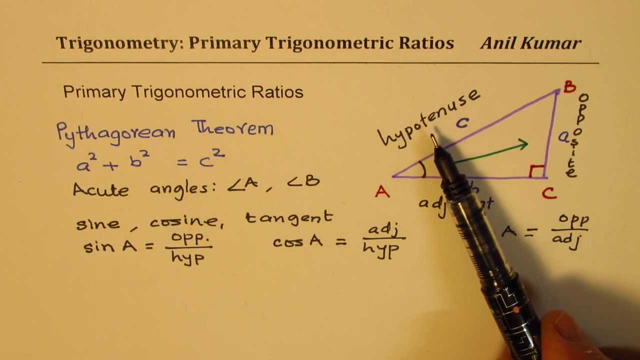 opposite side over hypotenuse And tan. the tangent ratio, in short, written with lowercase t, tan, tan A is equal to opposite side over adjacent side. So you can see from here that whenever hypotenuse is involved, we are talking about sine or. 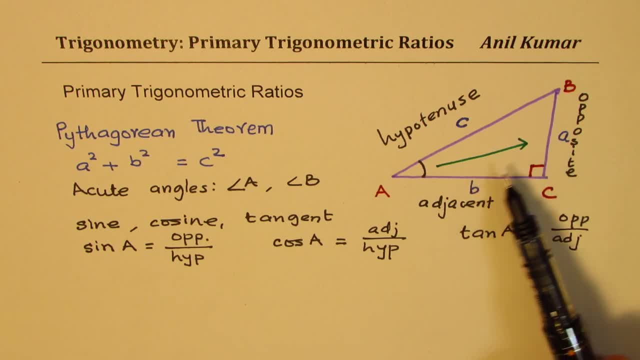 cosine, But if we are only considering two smaller sides, it is always the tan ratio. So most of the problems dealing with height and distance- Height and distance- will be solved using tan ratio. You get the idea right. So that is how we should treat it Now. here is easy way to remember. 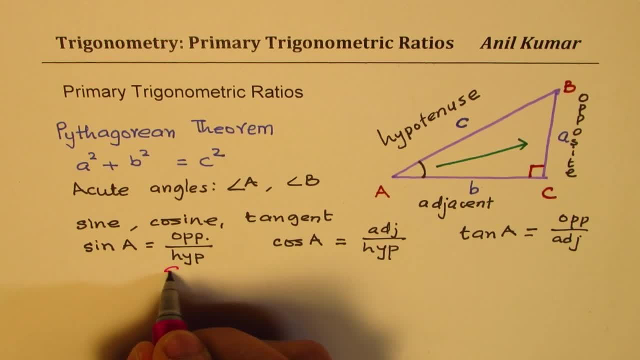 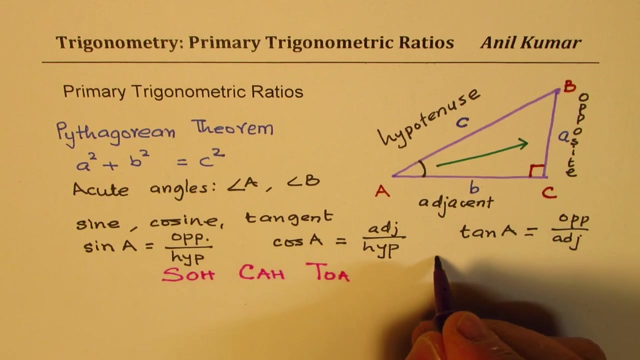 right. so so we say: sine is equals to opposite over hypotenuse, cosine is adjacent over hypotenuse and tan is opposite over Adjacent. some students remember: is SOH CAH TOA right? SOH CAH TOA. You may also write this in another form, just to remember which a sine is. 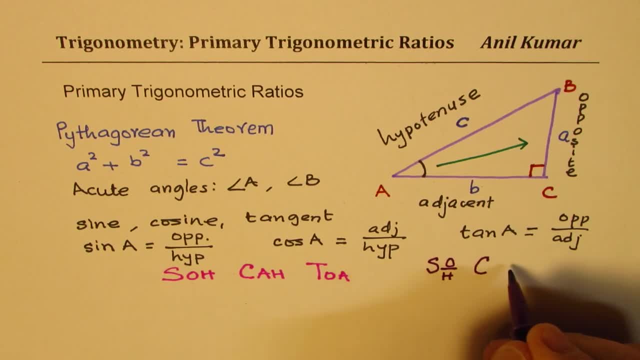 opposite over hypotenuse. cosine is Adjacent over hypotenuse and tan is opposite over adjacent. So that helps you to remember these ratios. Now I hope things are absolutely clear, right? So we saw these ratios from the point of view of angle A, Right, if I do angle B, then things change from angle B. 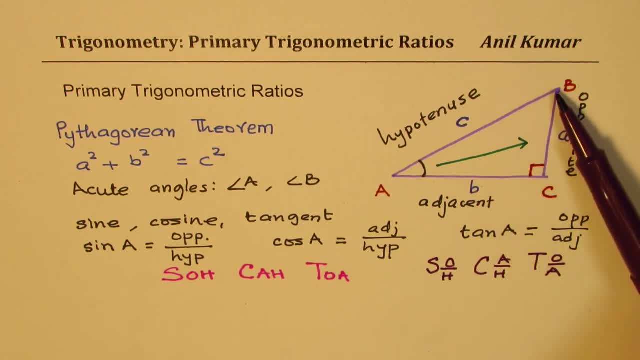 The opposite side is AC. Do you see that part? from angle B, The opposite side is AC. Perfect, So keep that in mind, Right? so sometimes we'll have questions where we'll talk about the angle, not the one shown here, but the other angle. 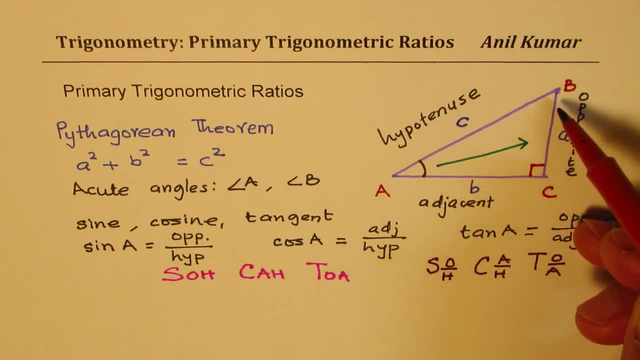 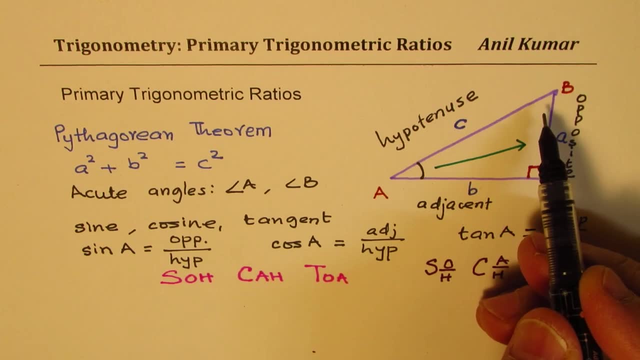 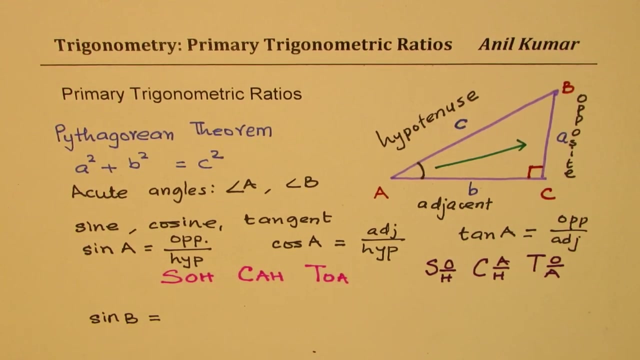 So you have to look into opposite and adjacent with reference to the angle. Now let us consider trigonometric ratios from angle B also, right? So if I write what is sine of B equals to Sine of B. if you see from the angle B, then the side opposite is: 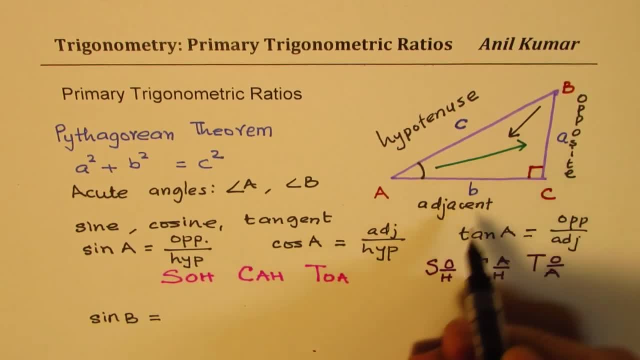 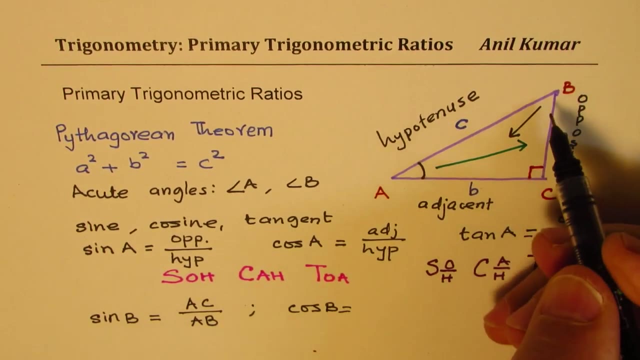 AC right. so it is a positive or hypotenuse Right. that's the definition opposite- over hypotenuse. Then it should be AC over the hypotenuse. AB: right Cos of B will be equal to. we are seeing from angle B now: right cos of B will be adjacent side. 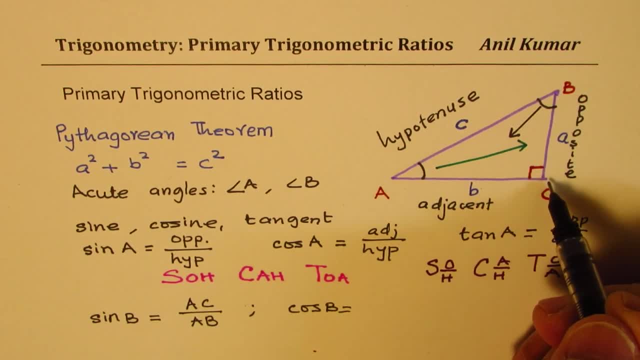 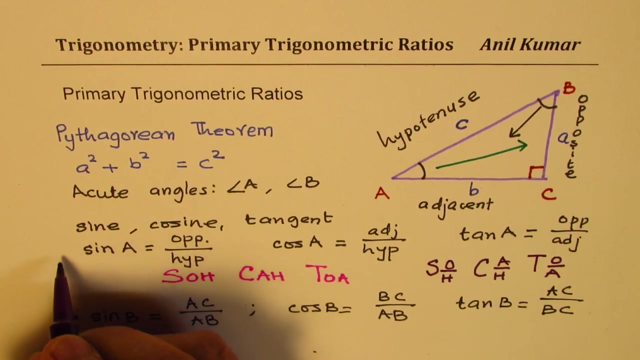 So the side which was opposite to a becomes adjacent. I hope you realize right. so it becomes BC over AB and tan ratio, Tan of angle B, will be AC over BC. So you clearly see that if we change the angles then things reverse, correct? So you could be asked to find trigonometric ratios from angle A or from angle B. 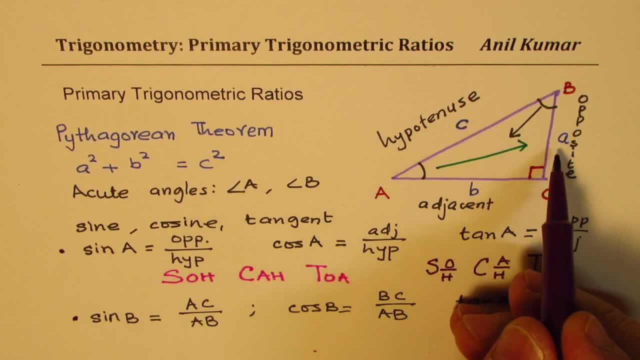 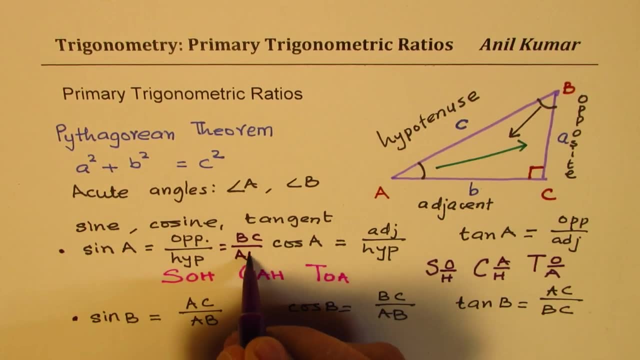 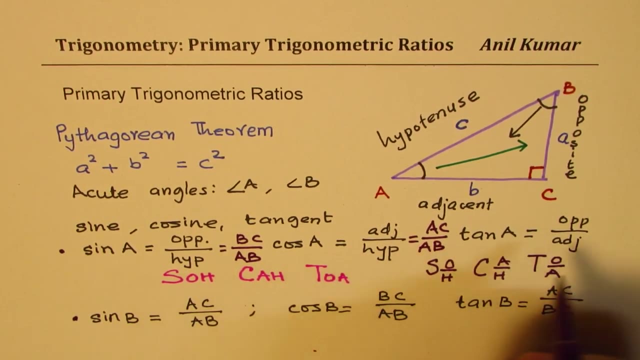 So, from angle a point of view, the opposite side is BC, so this could be written as: BC over AB, Cos, adjacent side AC over AB and tan opposite side BC over AC- Perfect, So I like you to have a good look at this sheet that gives you all what you need to do. 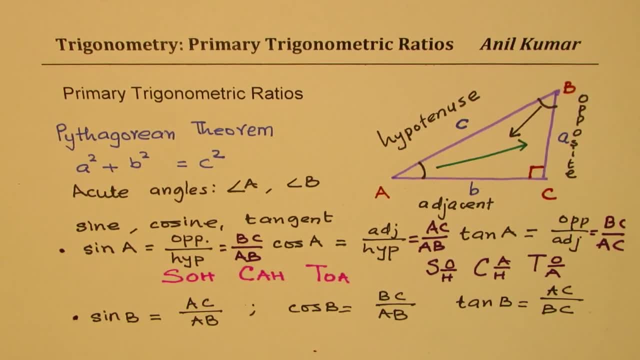 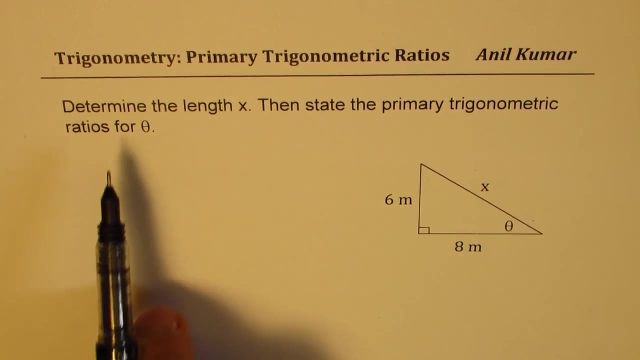 To solve the remaining six examples, and that should give you good practice. I hope you're ready, So let's begin and answer these questions one by one. So let us begin with our practice questions. Here is the very first one: Determine the length X. then state the primary trigonometric ratios for theta right. 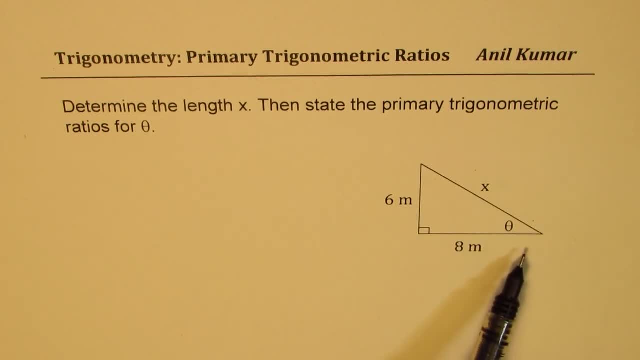 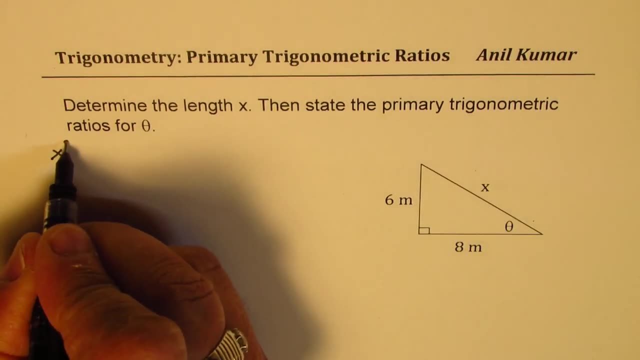 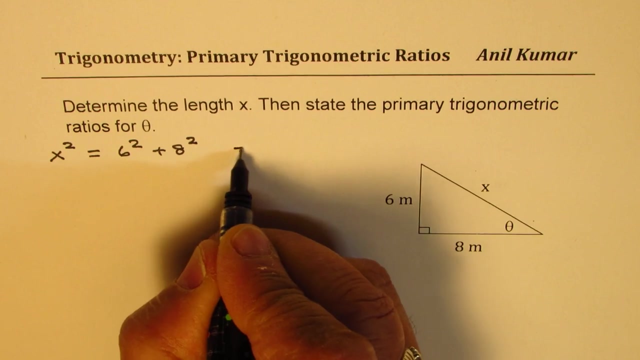 So the angle theta. to find X in any right triangle, the hypotenuse, we can add sum of squares of the other two sides. so using Pythagorean theorem we know X square is equal to 6 square plus 8 square right, which in our case is: 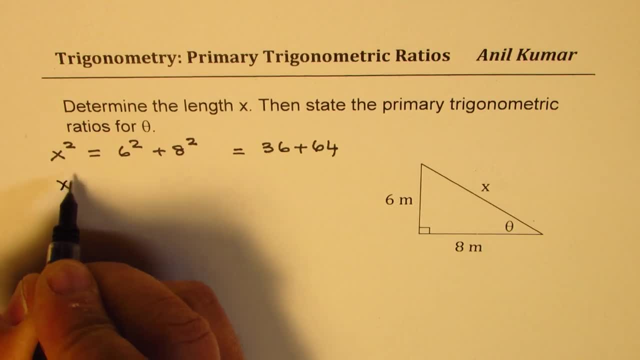 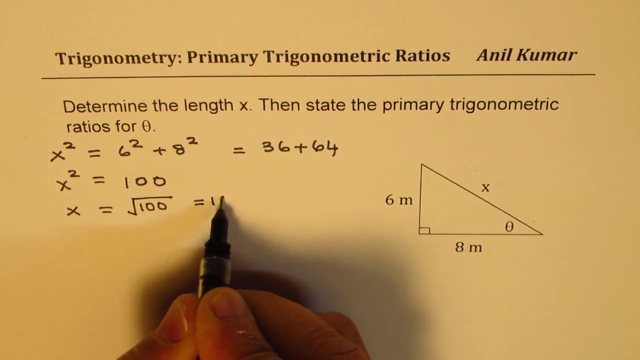 36 plus 64. so we know X square is equal to 100, right, 6 plus 4, 10 and Then 10, 100. So X is equal to square root of 100, Which is equal to 10. so purposely I've taken very easy numbers to work with, but they explain the whole concept. 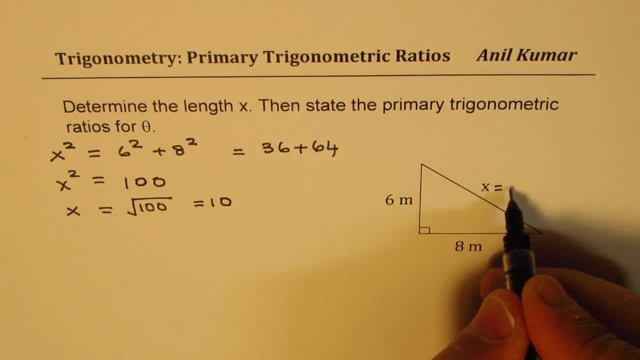 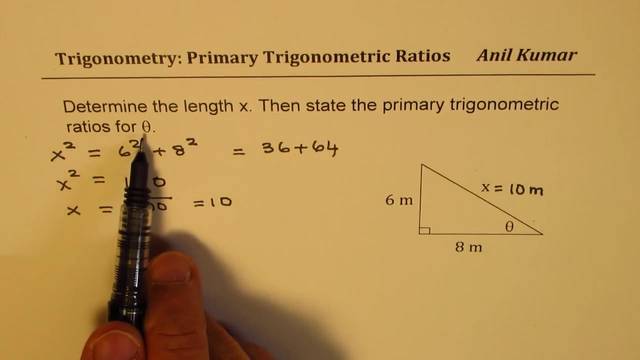 Perfect. So we found that X is equal to 10 and the units will be meters. Now let us find the primary trigonometric ratios for angle theta. so let us begin with sine theta, So sine of theta will be, if you're looking from: 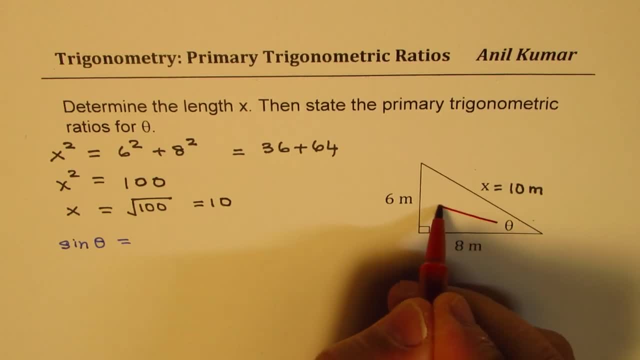 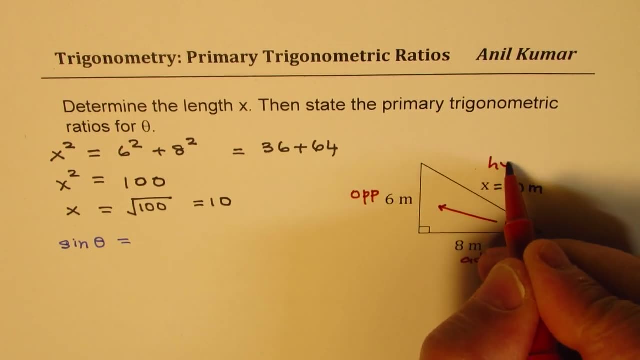 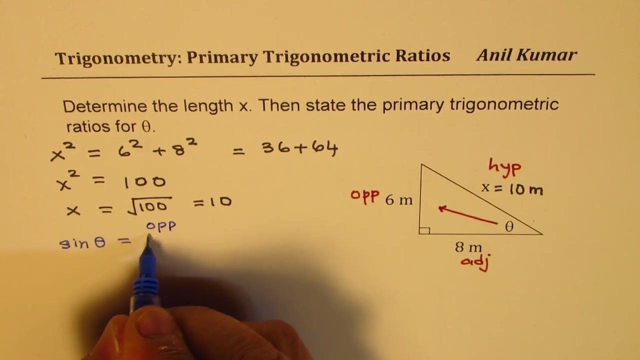 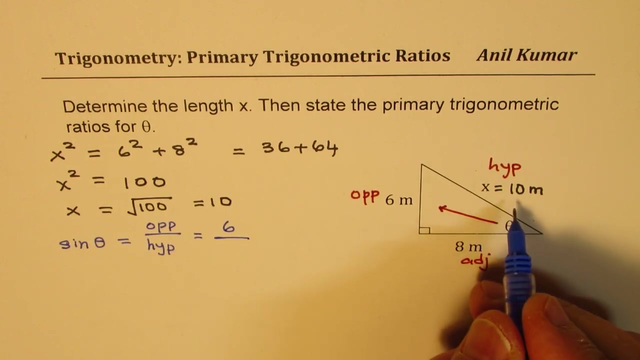 theta, this angle, then the side opposite is this: so this is your opposite side, this one is adjacent, and that, of course, will be hypotenuse. okay, sine ratio is the ratio of opposite side over hypotenuse. so in our case, opposite is 6 and the hypotenuse is 10, as you will notice. 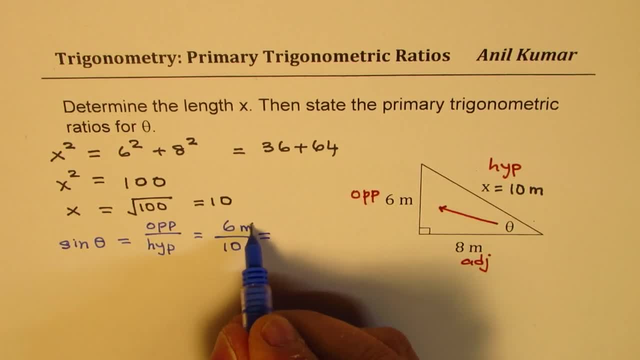 the units cancel. so even if i write meters and meters, they cancel. so primary trigonometric ratios are ratios. they do not have any units. you could not simplify this. dividing by 2, we get 3 over 5 as sine of theta. now this is the exact value, perfect, 3 over 5. let us find what is cos theta. 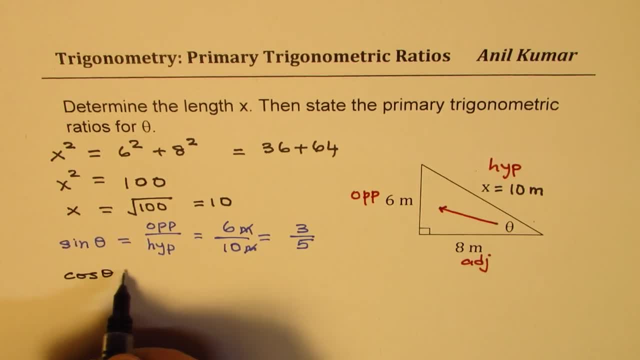 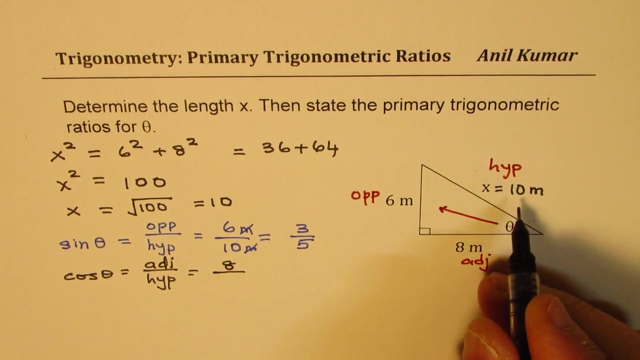 so cos theta is adjacent sine over hypotenuse. in our case, size side adjacent to angle and 90 degrees is 8 meters. so we'll write 8 here. forget about units now. okay, if you have the same units you can just forget, otherwise you may have to convert them to same units. so 8 over 10. this could be simplified and written in the: 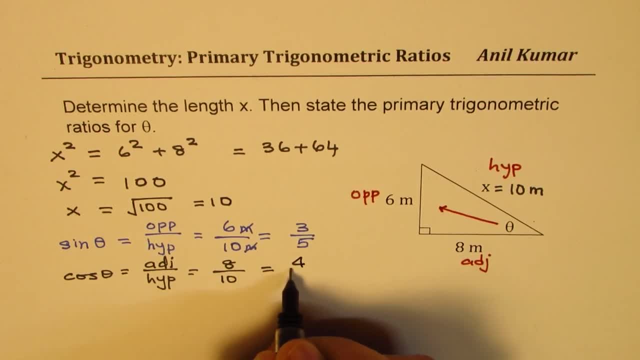 lowest form. dividing by 2, we get 3 over 5 as sine of theta. so this is the ratio of opposite side: 4 over 5 as the value of cosine theta. what is tan theta? tan theta is the ratio of opposite over adjacent right, is the ratio of opposite over adjacent side, which is 6 over 8. 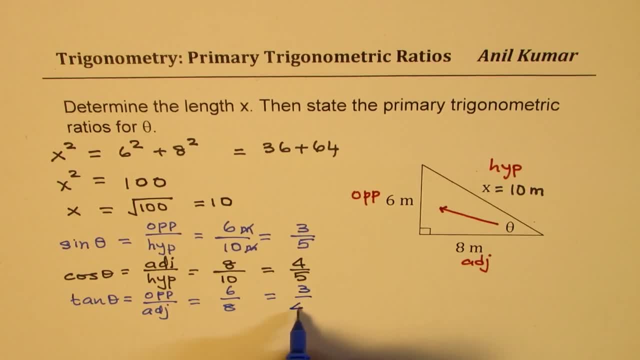 or 3 over 4. okay, so what you remember here is the ratio: sine is opposite over hypotenuse, cosine is adjacent over hypotenuse and tan is opposite over adjacent, correct? so cut over. so that helps you to get the results. so i hope it is absolutely clear. let's continue and take up the 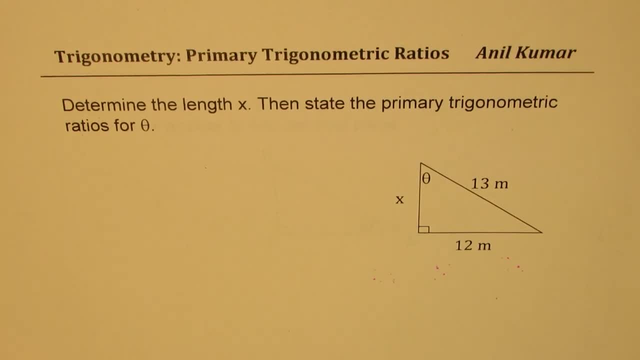 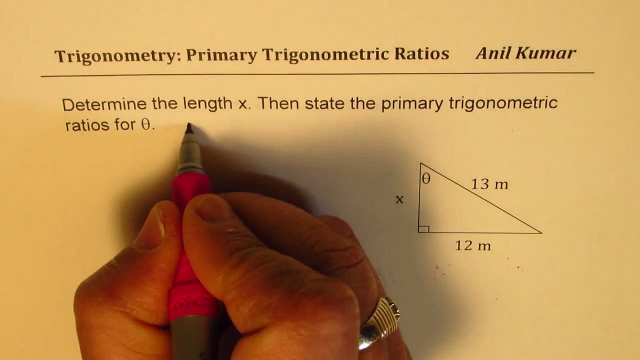 next question, which is very similar, right? so i like you to pause the video this time. answer the question and then look into my suggestions. we need to determine the length x, then state primary trigonometric ratios, right, so you remember. so cut over so you may write here to begin with. 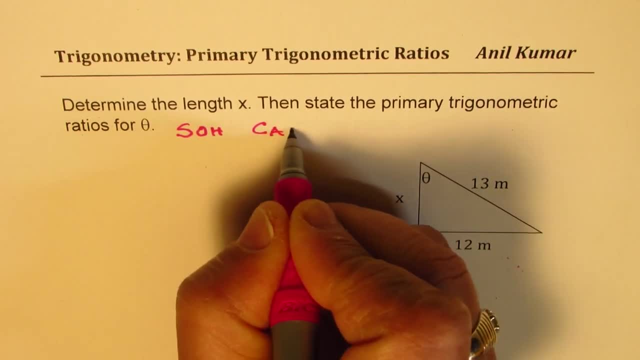 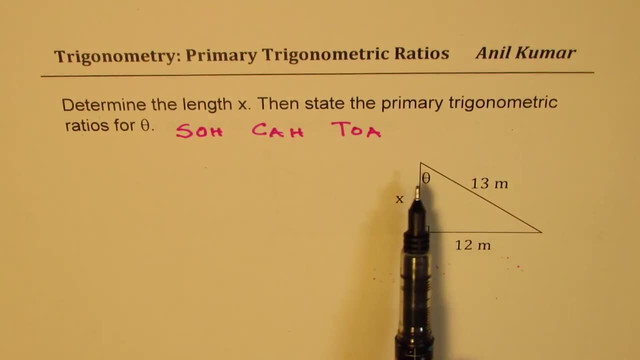 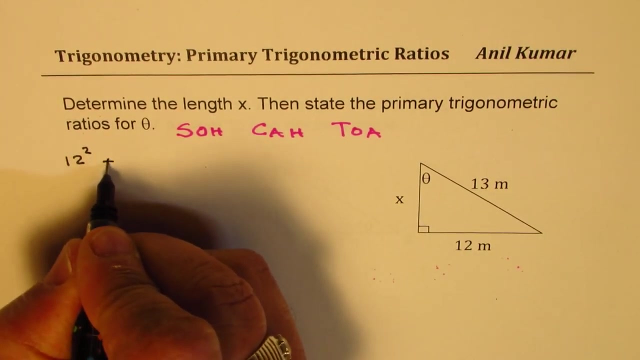 sine is opposite over hypotenuse cosine, adjacent over hypotenuse tan, opposite over adjacent right. but we need to first find x. now this is a smaller side, correct? so in this case we know 12 square plus x square should be equal to 13 square. so that means that x square should be equal to 13 square. 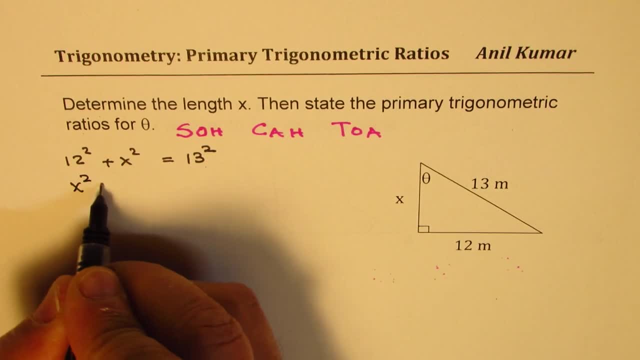 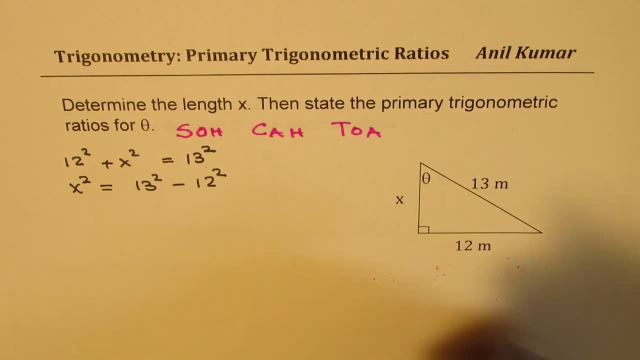 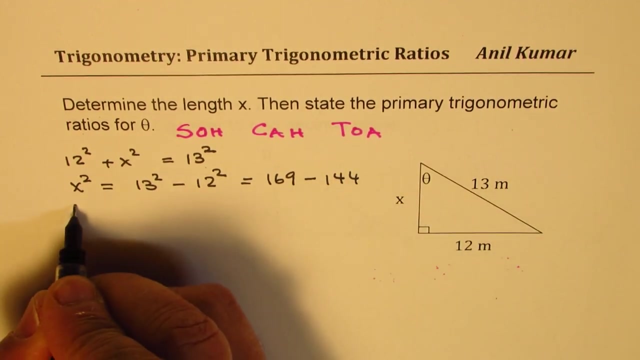 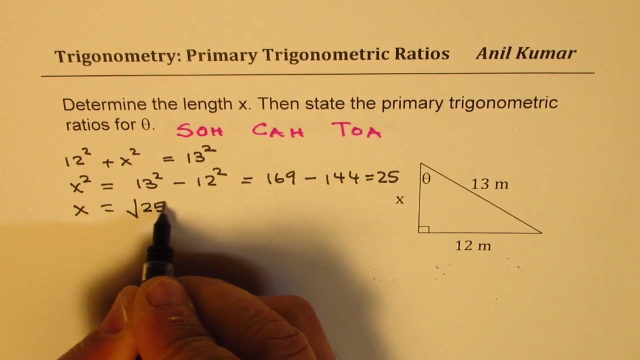 so that means that x square should be equal to 13 square. so that means that x square should be equal to 13 square minus 12 square. so so you can say this is equals to 169 minus 144. use calculator, okay. so x is equal to, which is 25. so x is equals to square root of 25, which is equal to 5. so the 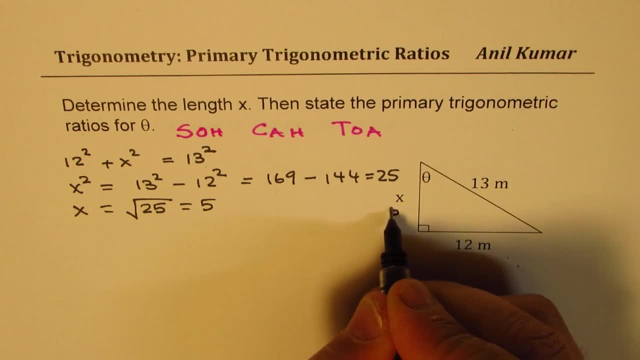 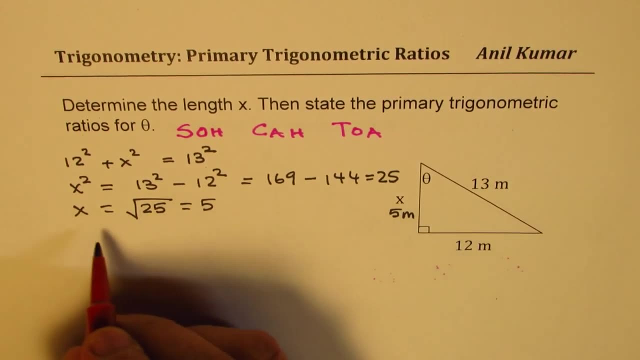 side, this length is equal to 5 meters. perfect. so that is the first part. so we are done with finding all the sides of a right triangle. now the second part is to write down the ratios. so let's begin with sine. sine of the angle, theta is equal to what it is equal to opposite side over hypotenuse. now, in our case, the side opposite. 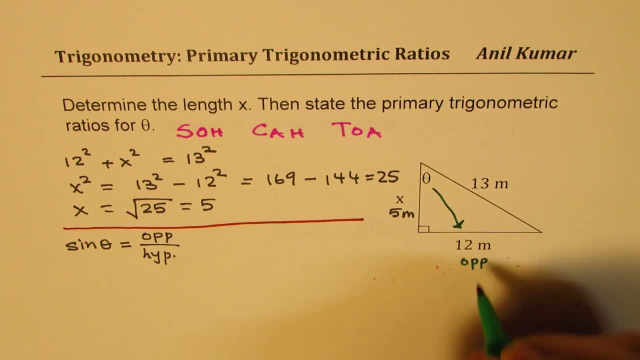 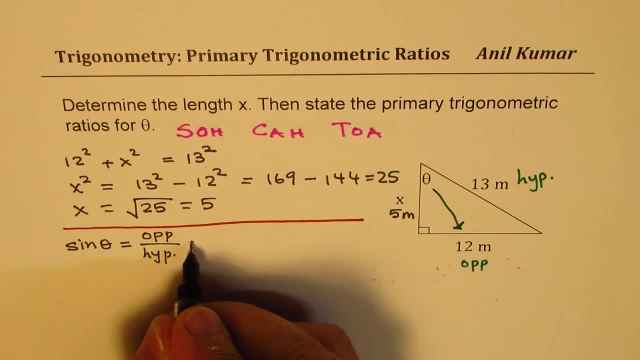 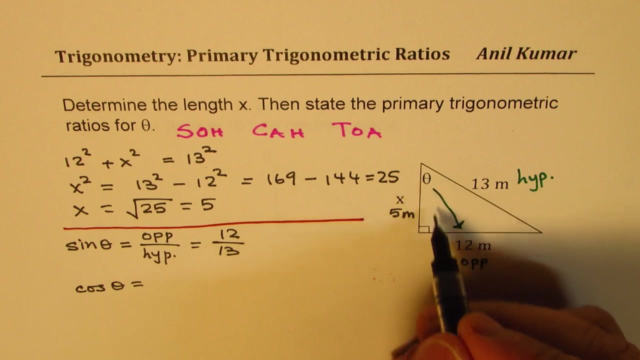 to theta. is this side right? this is the opposite side, and here we have hypotenuse. therefore this ratio should be equal to 12 over 13. clear. now let's write down what is cosine of angle theta. adjacent side is the side here between the angle and 90 degrees, 5 meters. 5 divided by the hypotenuse 13. so that gives you. 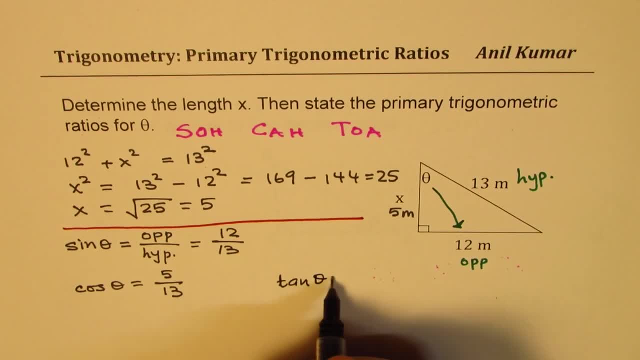 the answer for cos and for the cosine of the angle theta. so let's write down cosine of the angle theta. and for tan theta we could now directly write opposite over adjacent, which is 12 over 5. is that clear? so that is how you could write your ratios. now it is not necessary that you always write opposite. 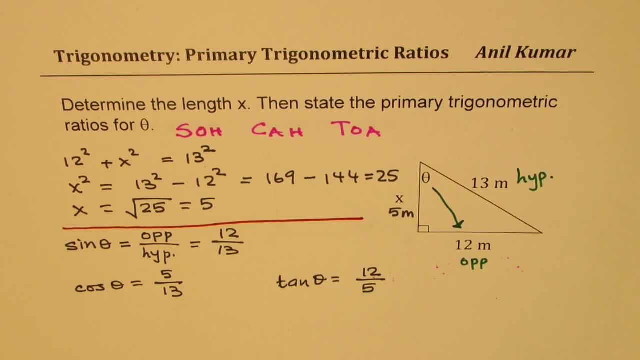 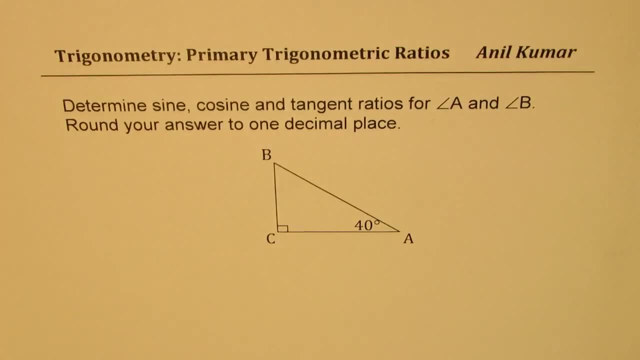 over hypotenuse. this is for you to remember. now, since we are assuming this is these examples as one of your first exercise, we are repeating it. okay, here is another question which is very much related to our previous example. determine sine, cosine and tan ratios for angle a and b round your 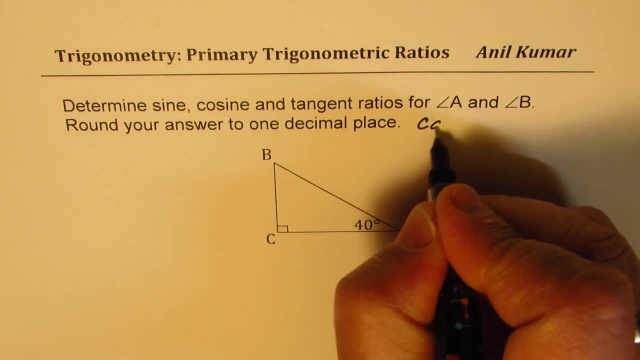 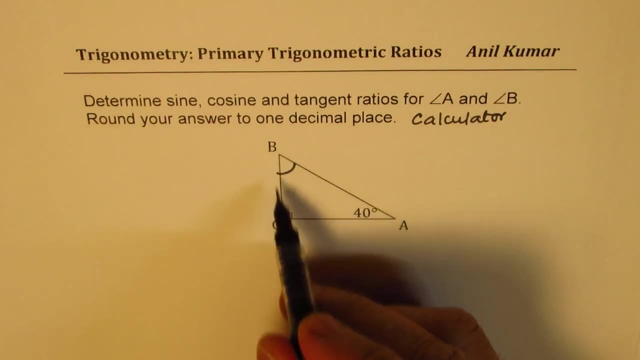 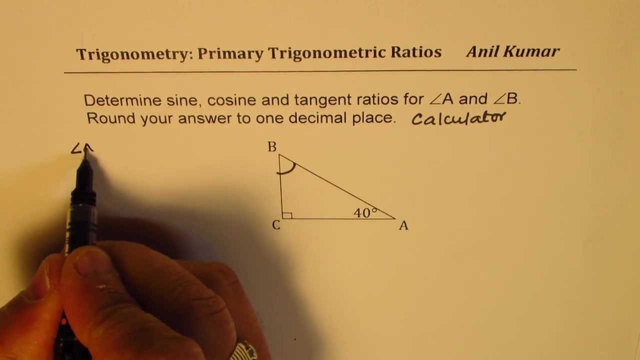 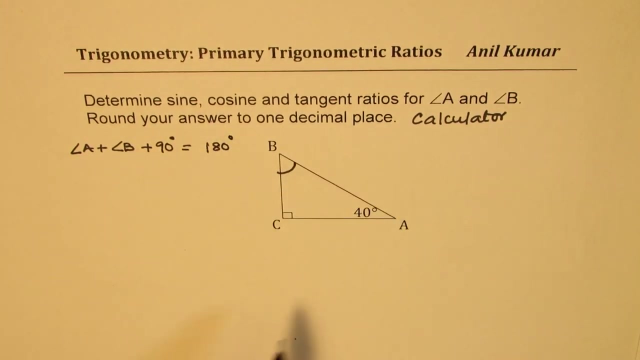 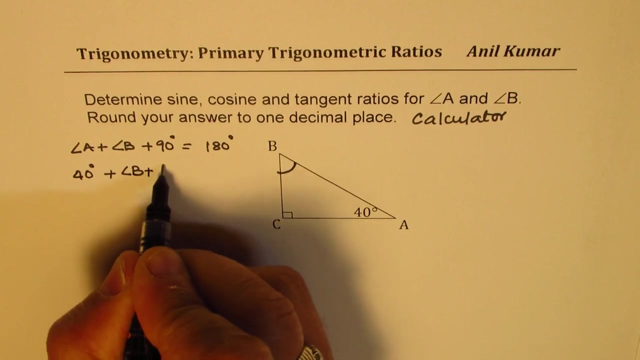 answer to one decimal place, so we need to use calculator here. first part is to find angle v. now, in the sum of all these angles is 180 degrees, right? so we can say that angle a plus angle b plus 90 degrees is equal to 180 degrees. we know angle a is 40, so 40 degrees plus angle b plus 90 degrees. 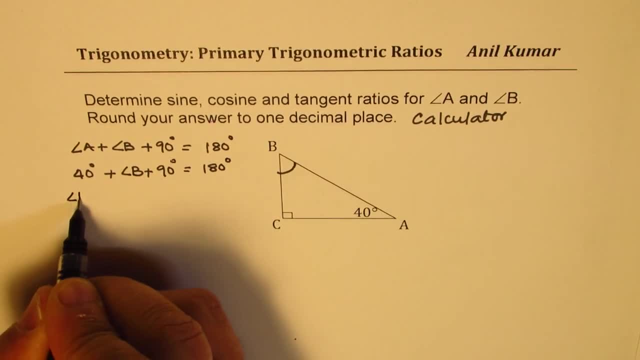 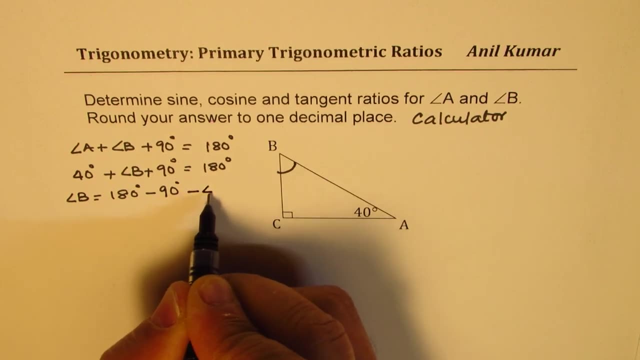 is equal to 180 degrees. so we can find what is angle b from here, which is 180 degrees minus 90 degrees. that is 90 minus 40 degrees. that gives us 50 degrees. so angle b is 50 degrees correct. you may use calculator to find. 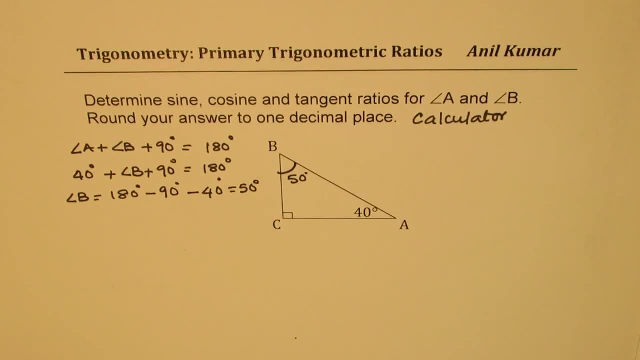 this: once you know all the angles, then we can find sine, cosine and tan of angles, the acute angles, using calculator. so let's find for angle a, which is equal to 40 degrees, first right, and then we'll calculate for angle b, which is equal to 50 degrees, using calculator. so so, using calculator, we can. 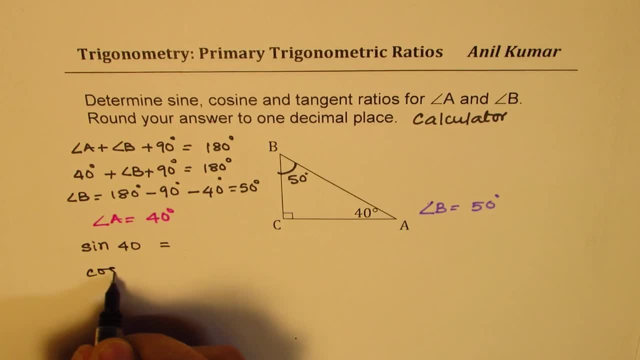 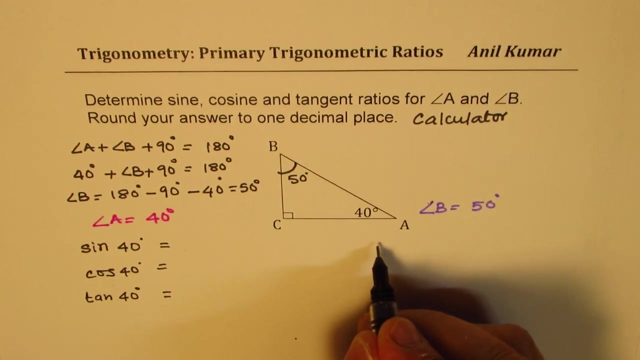 find what is sine of 40 degrees, what is cosine of 40 degrees and what is tangent of 40 degrees. we need to round these answers to one decimal place. similarly, we'll also use calculator to find sine of 50 degrees, cosine of 50 degrees and tangent of 50 degrees. these three are called the. 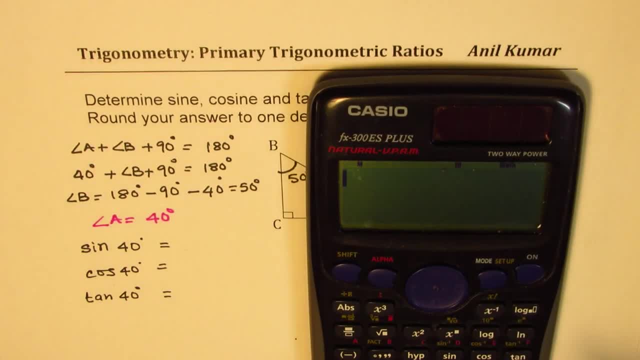 primary trigonometric ratios. so the setting should be in degrees, which is the default setting. when we say sine of 40, then press sine and then the angle. you may have to close the bracket at times. right, it should be done. normally you have to put the angle in brackets, so one bracket the open. 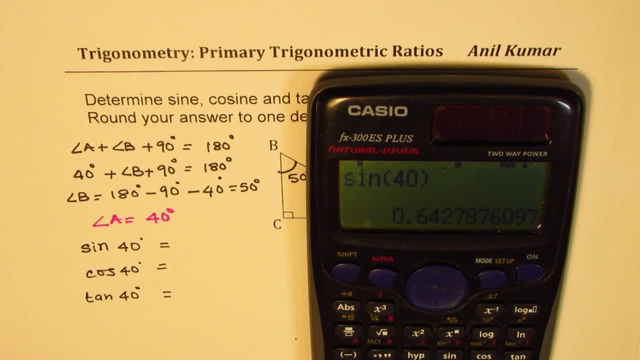 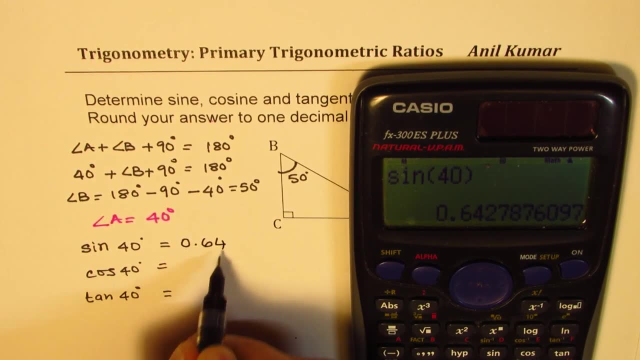 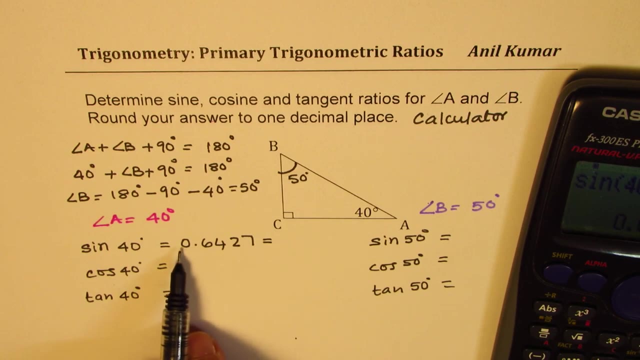 bracket is given by default. you have to close the bracket, press equal to write down the answer. it has to be less than one, right, so it will be zero point six, and then you have to write down the answer. so that is zero point six. four to seven: we need to round our answers to one decimal place so that 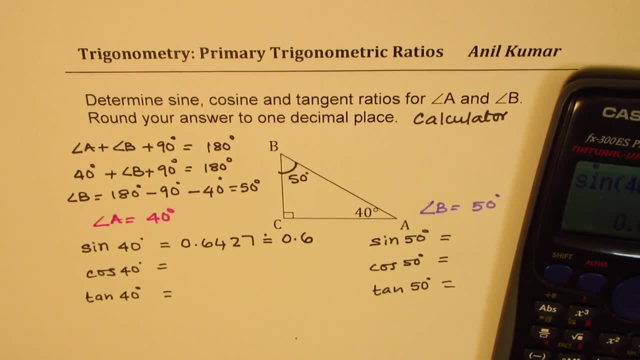 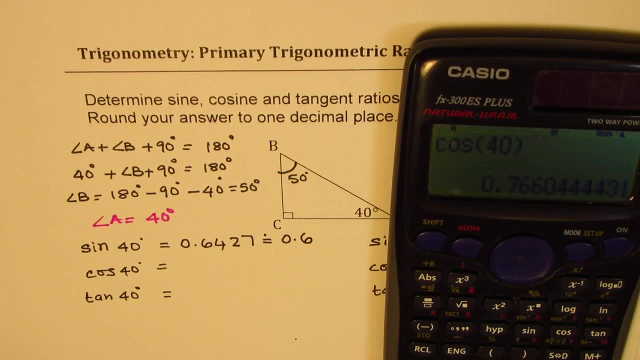 means I could write this as zero point six, right? so that is how you have to write your answers. so use your calculator and write down the answers. here are rest of the answers. cosine is zero point seven. six, six rounding, we get zero point eight. and for ten: 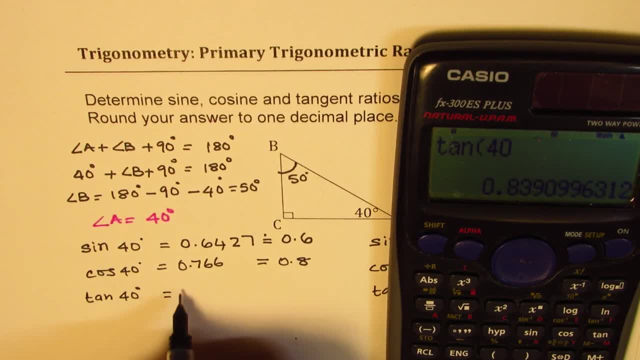 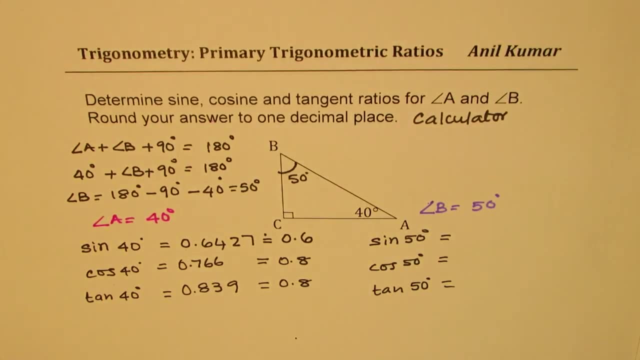 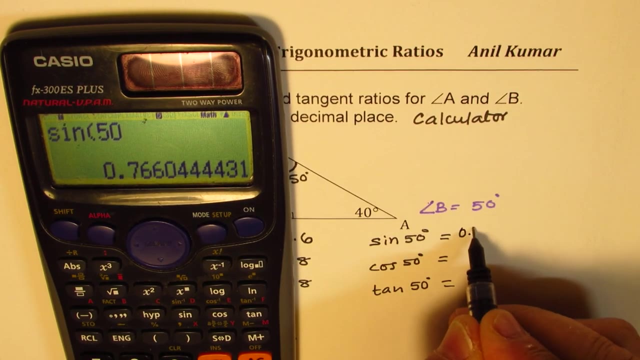 40 equals to 0.839.. Rounding gives me 0.8, right For sine of 50, we'll do sine. 50 equals to 0.766, which is 0.8.. I should have done it in two decimal places, then you would have seen more difference. 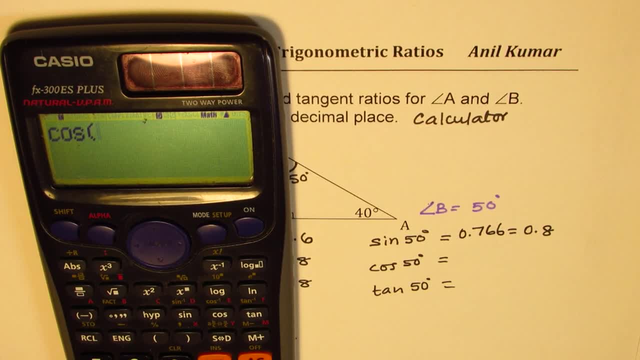 right. Anyway, cos of 50 degrees is equal to 0.642, rounded to 0.6, and tan of 50 degrees is equal to 1.191.. So tan ratio could be bigger than 1,. right Round to one decimal place gives me: 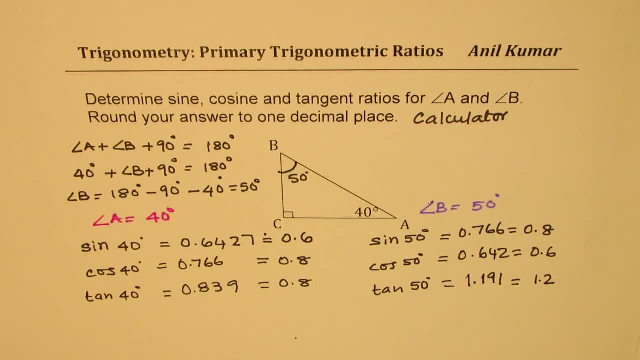 1.2., 1.2.. Now, what you notice here is a very important thing. that is, if you look from these sides, when we reverse the angles, sine of 40 is same as cos of 50. Do you notice that? 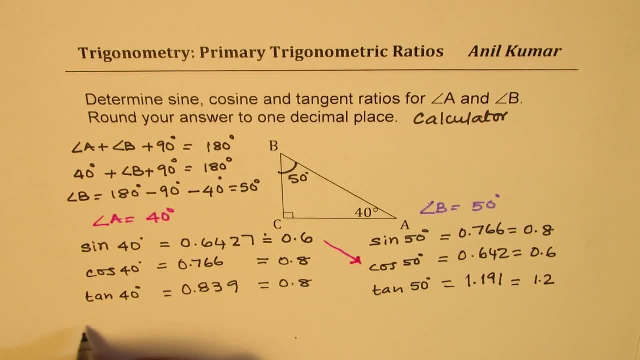 Sine 40 is equal to cos 50, right. So, important note, Sine 40 is equal to cos of 50.. 40, right. And we also notice that sine of 50 is equal to cos of 40, cos of 50, correct. 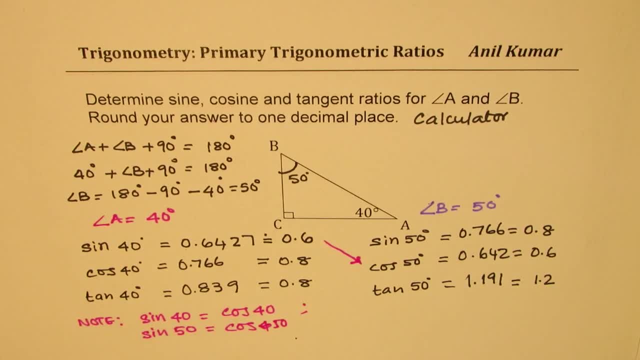 So sine of 50 and cos of 40 are also same. Do you see These are also equal, correct? Can you explain why? So that is your question: Explain why. Okay, So let's move on And take up next example. But I hope you have understood some very basic concepts with this. 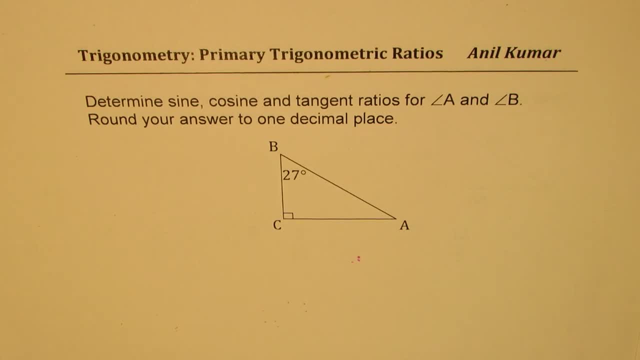 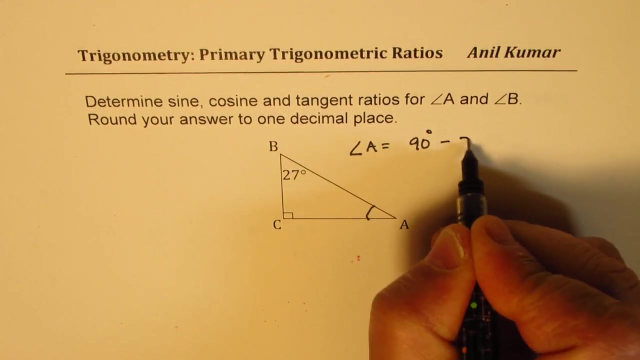 example. Now again, it is a similar exercise. You are again given a right triangle with one of the angles. So first step is to find angle A. So what is angle A? So angle A could be written as 90 degrees minus 27 degrees. Do you see? You don't really have to write 180 minus 90. You know. 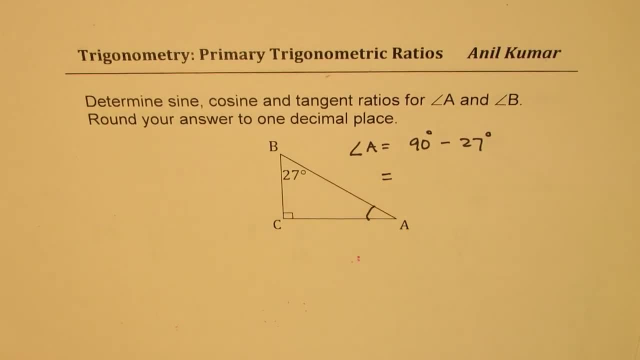 that is 90, correct. So at times you could save time. So 90 minus 27, you could do right. So 90 minus 27 is equal to 63.. So we get this angle as 63 degrees. Now you need to use your calculator and write down the. 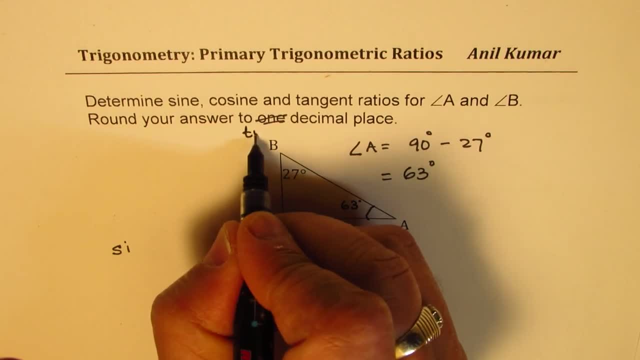 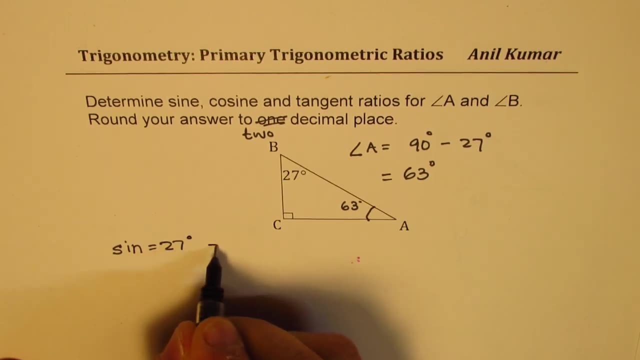 answers. So this time we'll change it to two decimal places, okay, So write down sine of 27 degrees, cos of 50,, cos of 50, and then write down the angle A. So you have to write down the angle A, So. 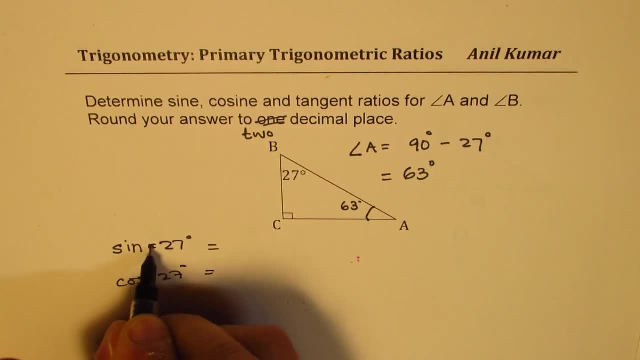 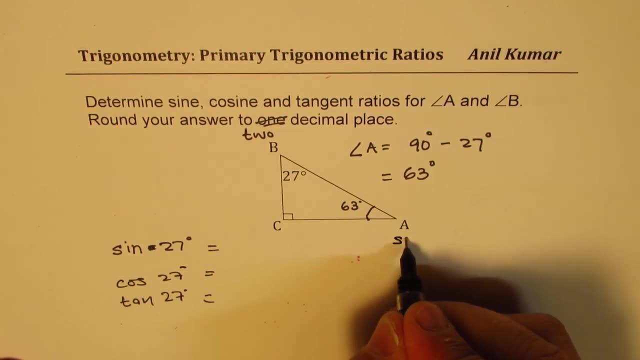 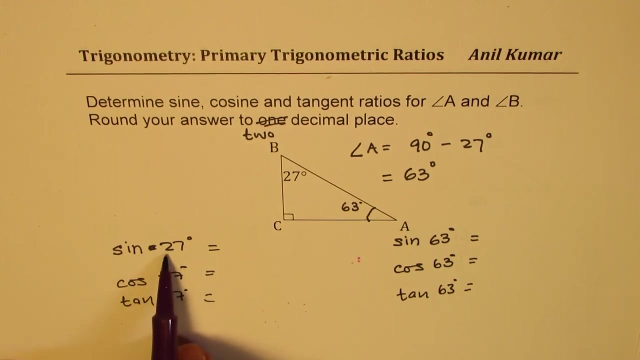 27 degrees and tan of 27 degrees using calculator, and also calculate sine of 63 degrees, cosine of 63 degrees and tan of 63 degrees. also, you will notice that sine of 27 is equal to cos of 63.. so again, use your calculator. write: 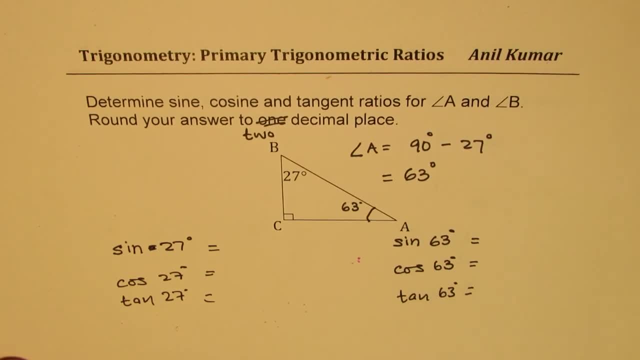 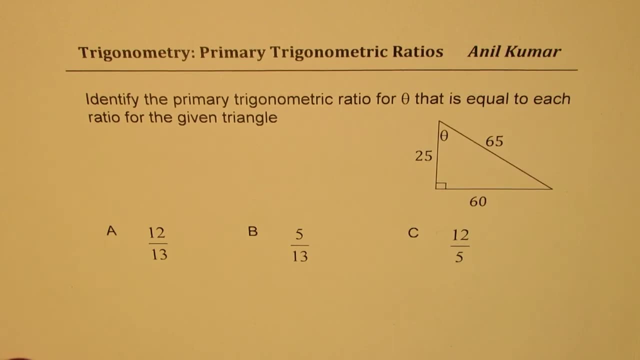 down the answers. so I leave this exercise for you to completeI hope that makes sense. Now here is the last question: identify the primary trigonometric ratios for theta. that is equal to each of the ratio given. so you are given the ratios 12 over 13,. you have to. 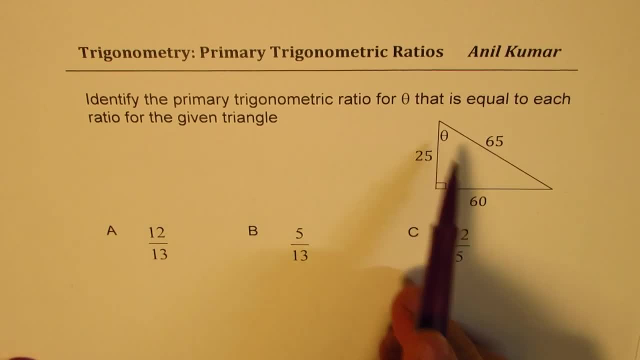 identify. identify whether it is sine theta, cos theta or tan theta. perfect, so you can pause the video, answer this question and then look into my suggestions. remember, sine is opposite over hypotenuse, cosine is adjacent over hypotenuse and tan is opposite over adjacent. so from this angle,